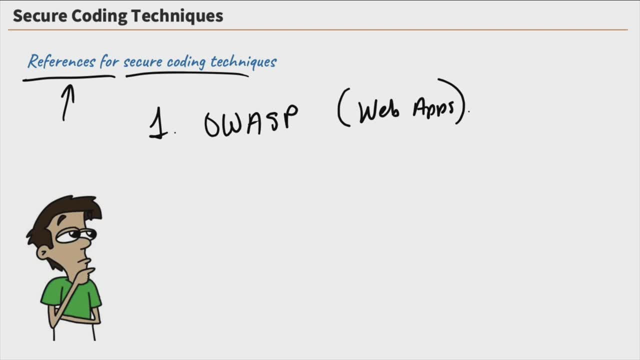 talk about some common web application vulnerabilities and such. So we're going to do that in the next series called Application Security and Software Assurance. Another resource is the ASVS, And that's the Application Security Verification Standard, The ASVS, And then, lastly, we have Software Assurance. 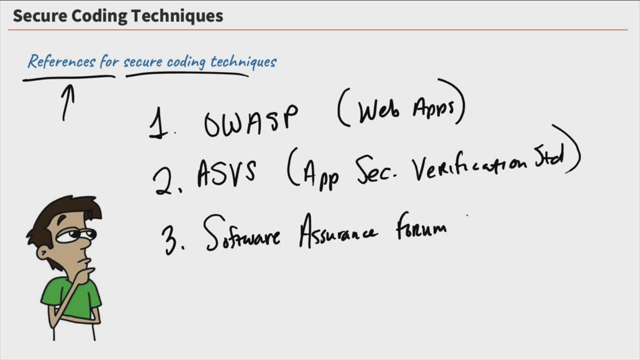 Forum for Excellence in Code, aka SafeCode. Those are three different resources that you should be aware of that provide us with secure coding techniques, So you can go out and you can Google them. You can go to the websites and they will provide you lots of information about how to 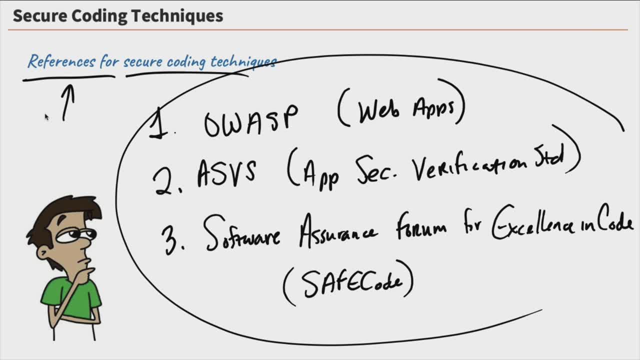 secure coding techniques. And then, lastly, we have Software Assurance Forum for Excellence in Code And some of them, like the OWASP, actually go out and they list out many common vulnerabilities And then they show you how to code properly so that those vulnerabilities don't show up in your code. 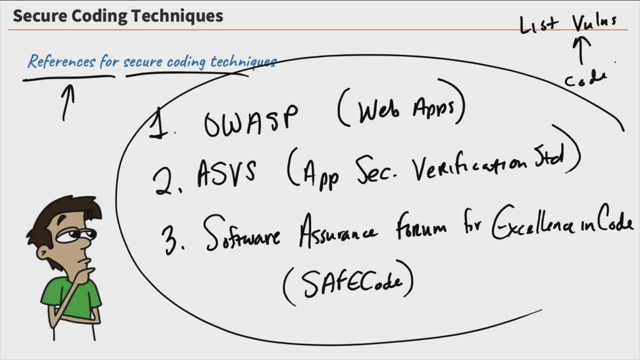 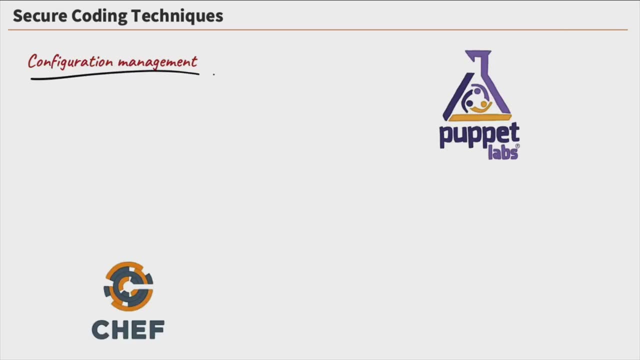 and your applications. So these are some great resources. Now, part of secure coding is also configuration management and versioning, So let's jump over to configuration management and take a look. So configuration management, what that is? it is a super important part of coding as it allows us to. 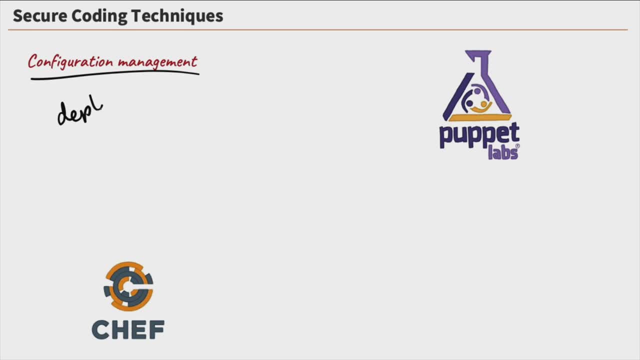 deploy standardized pieces of code. So we'll say: deploy standardized code. That is super important because if we can standardize our code throughout our environment, then we can know that it's all done the same way and it follows the same standards and it's all going to be secure. 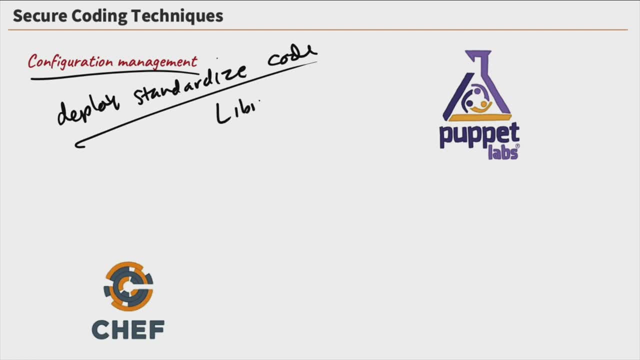 So really, what we can end up doing is creating a library of code pieces and then we can deploy from that library, because we know everything in this library is secure code, And there's two very popular tools that can be used to do this. The first one is Chef down here Now. 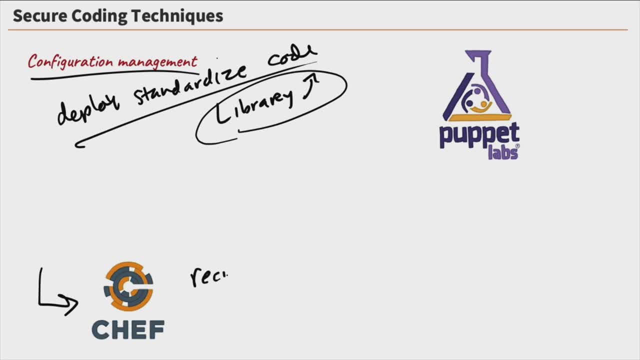 Chef configurations are stored as recipes. That's pretty cool. So these recipes can be used to automate the building and deployment of infrastructure components. So really, we take these recipes and we can automate deployment with them. So, really, what it is, it's a template. We're creating a code configuration template and that. 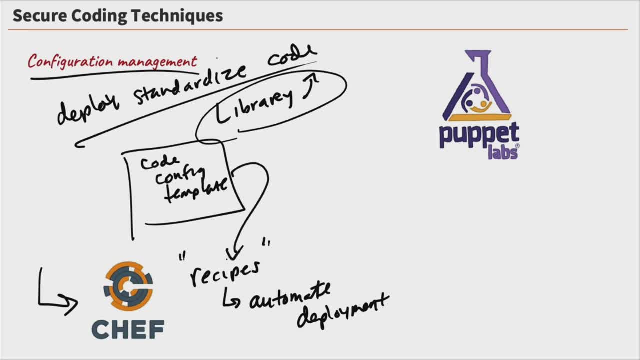 template is saved as a air quotes here recipe And then we can use that template to deploy infrastructure components. So that is Chef. That's the first one, And the second one is Puppet. that we're going to talk about quickly, And Puppet works by allowing you to define what you want. the state, 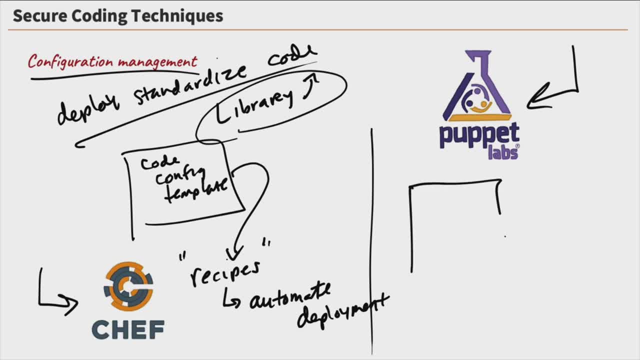 of your environment to be right. So basically, we're going to say: I want my environment to be like this And you kind of go through and you set really a bunch of settings. You're setting configurations, So here I'm setting: I'm going to use these type of passwords, I'm going to use this. 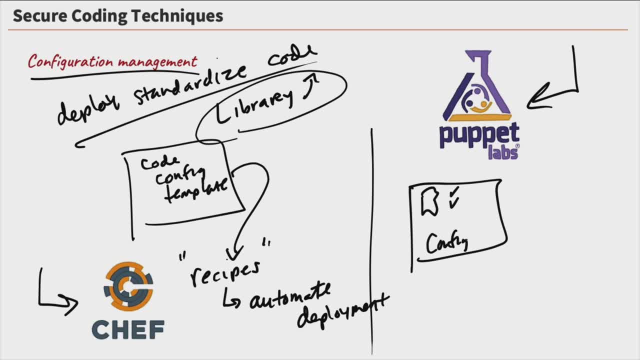 NTP server. I'm going to use these settings within my environment And then Puppet will go out and visit all of your assets out there that you have and make sure that they all meet this configuration policy, So they all match your desired state. So that is Chef and Puppet and configuration management. 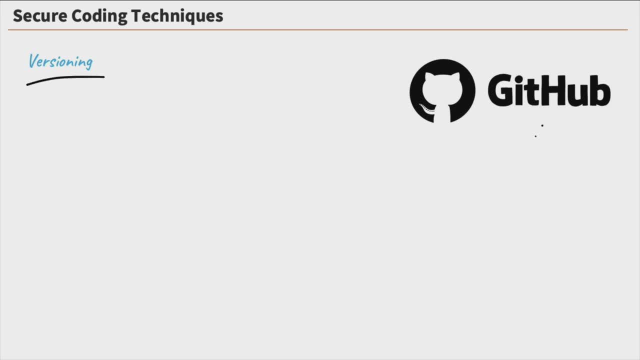 Next up versioning. Now. GitHub is a very popular tool in order to practice versioning, And the idea is that developers are devs out there. They use a repository, AKA repo, to store their code right. So a popular one is GitHub, And this really comes into play when you're using a team of people, as 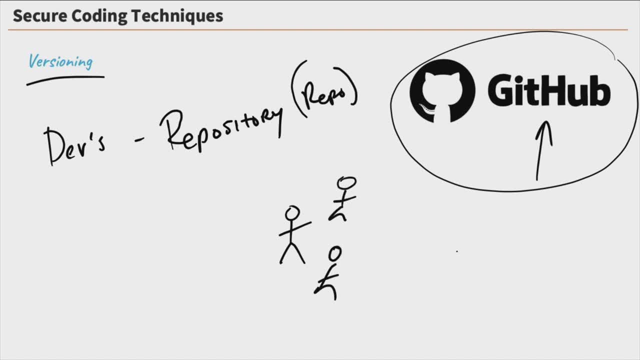 well. So you've got a bunch of devs out there and they're working away and they have this repo, GitHub and they store all their code. So you've got a bunch of devs out there and they're working away and they have this repo, GitHub and they store all their code. 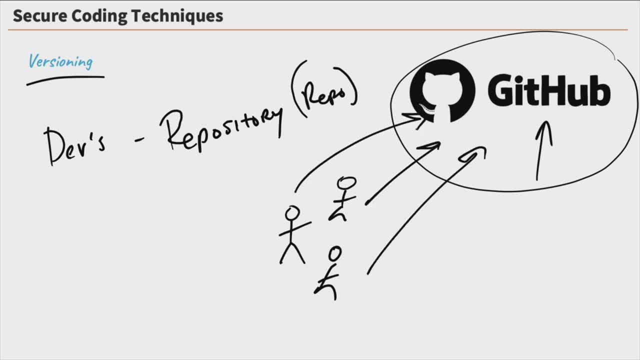 up here And they do it for specific reasons. One instance is when you're using a code repository. we'll say we've got our code up here in different chunks and somebody pulls down this piece of code right here. Well, it actually kind of puts it into a locked state. They've checked it out of the environment and now they're working on it, And that lets anybody else know who goes to access this code. 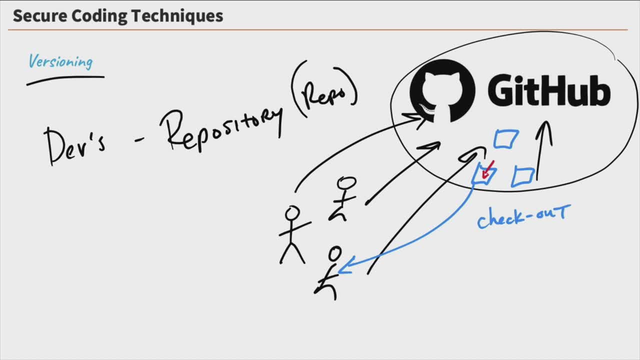 Hey, somebody's already checked this out and they're working on it, so that we don't have two people working on it and we end up with two different versions of the same code at the same time. That can cause some confusion And when this user is finished working on it. 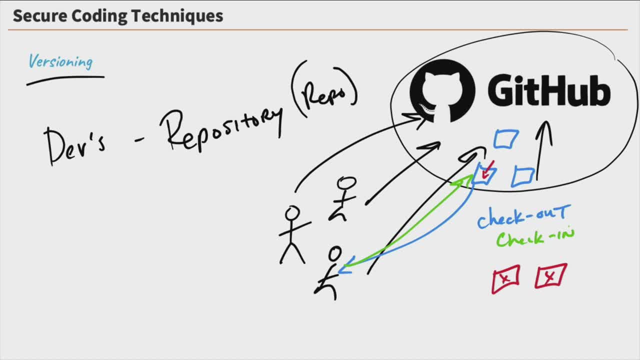 well then, they're going to check it back in and it's now back in the repository And each time these are checked out and checked in, we have version numbers assigned to them, so that we have versions and we can actually go back and look at previous versions. 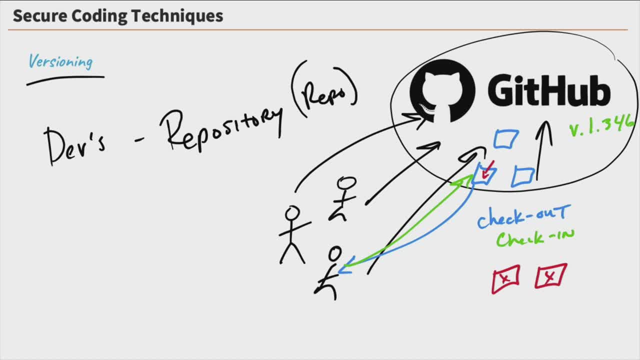 So if somebody edits a piece of code and then it messes it up, well, we don't have to worry about it because we have the previous versions. And that's the idea of versioning. And those are some of the secure coding practices. 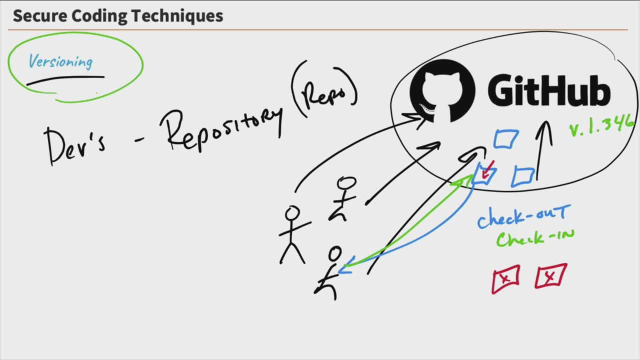 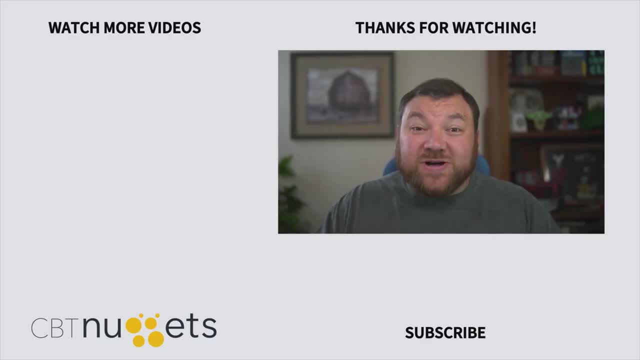 that we need to be aware of, especially when it comes to developing code in the cloud. I hope this has been informative for you and I'd like to thank you for viewing. Thanks for watching and subscribe here to get the latest from CBT Nuggets. 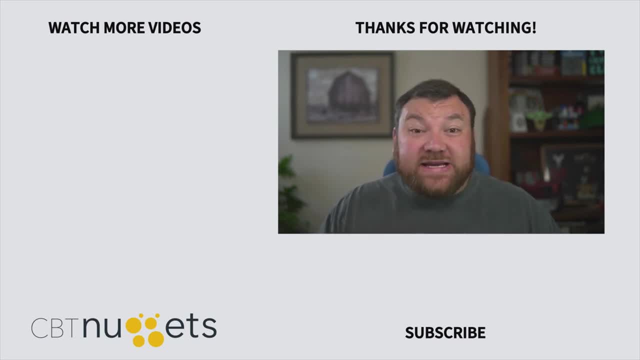 And if you're interested in IT career or learning more about IT in general, hey swing by cbtnuggetscom and sign up for a free trial. Thank you. 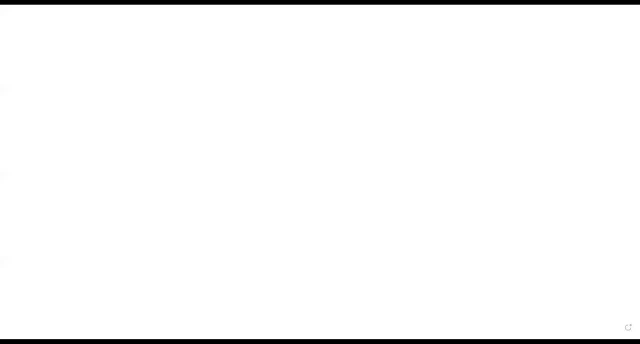 A relay. What is a relay? 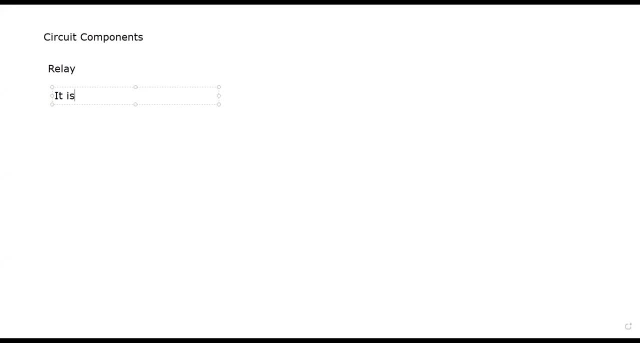 Relay is basically it is electromagnetic switch. The circuit symbol for the relay. 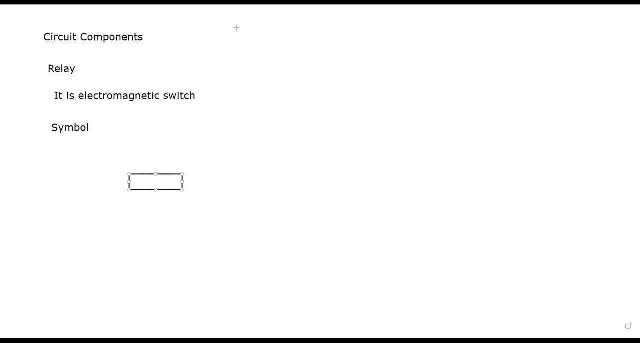 So how we represent a relay, a rectangular box, which is showing an electromagnet. And. And open the relay. And open the relay. And switch. 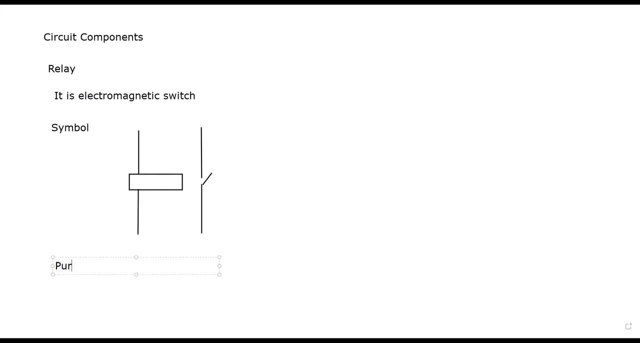 What is the purpose of the relay? It is used to connect. High current circuit. 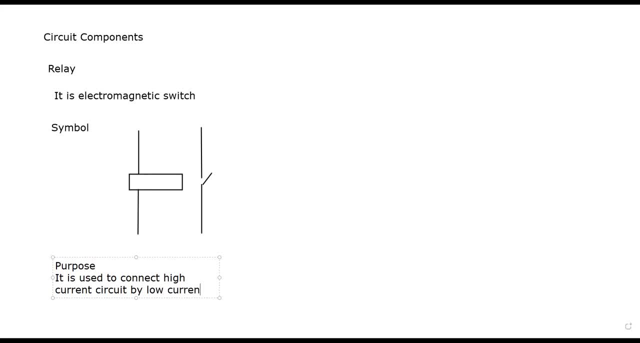 By. Low current circuit. Safe. High current circuit. For high current circuit. 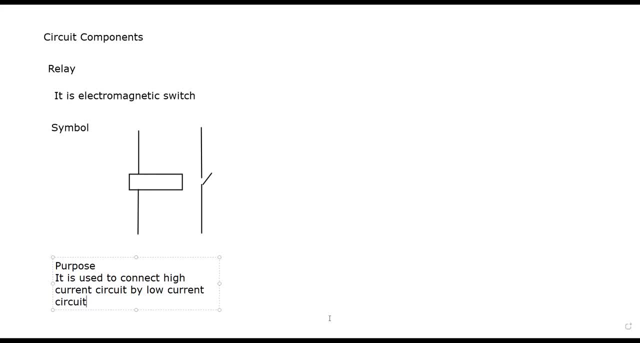 I don't expect that. Got it. Okay. 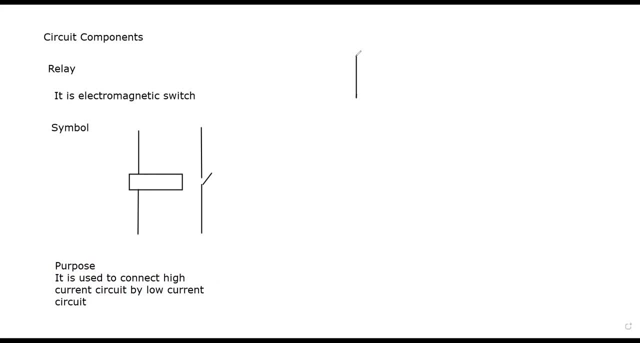 So for example. For example. Any. Could have. That would be. A little faster. Can you see what it means you have. The end gate. czne. It does the. Can you see the output? Let me get it. And get.